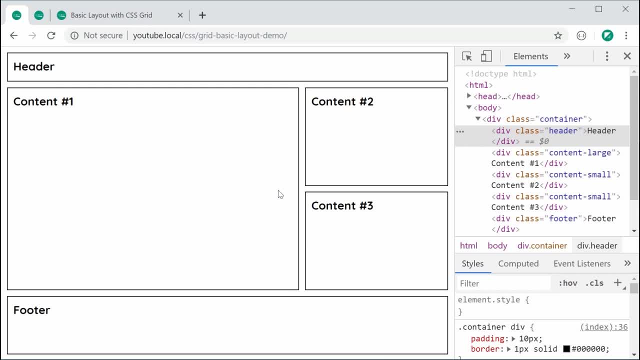 I'm going to be covering most of the main features so that you can get started and, of course, start implementing CSS Grid for your own web projects. So this, right here, is a basic layout. We have a header, we have some content sections and we have, of course, the 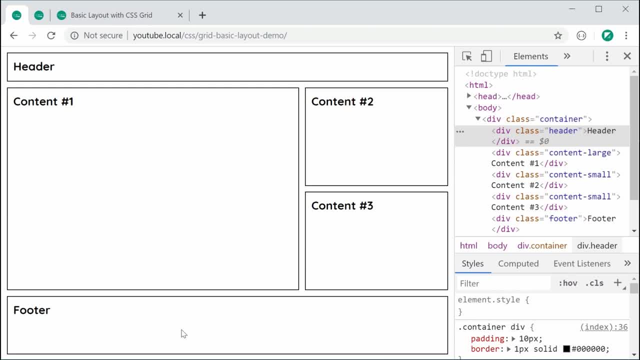 footer. So basically, this layout is going to support this right here. So this sort of 2 column content layout as well as a 3 column content layout, just like this. So there's a small change in the CSS in order to transform this right here into this right. 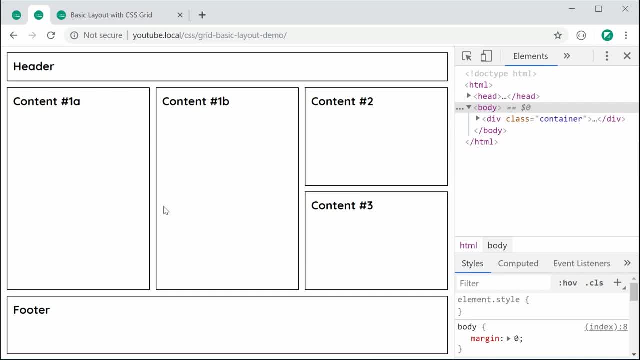 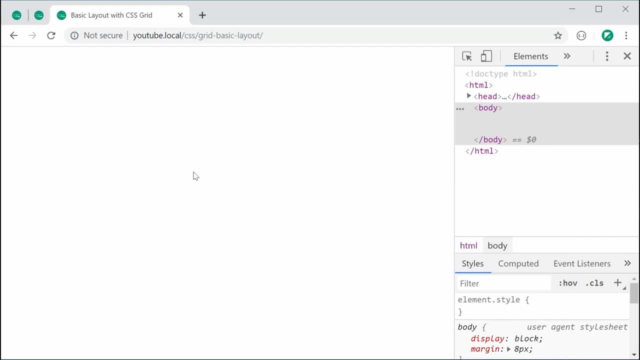 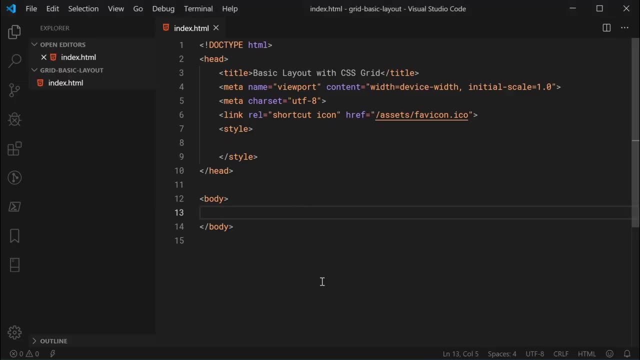 here. So of course you can choose which one suits your scenario better. So anyway, let's go inside this HTML file right here. We're going to start from scratch to create that layout. So inside the text editor it looks something like this: It is a plain HTML skeleton. 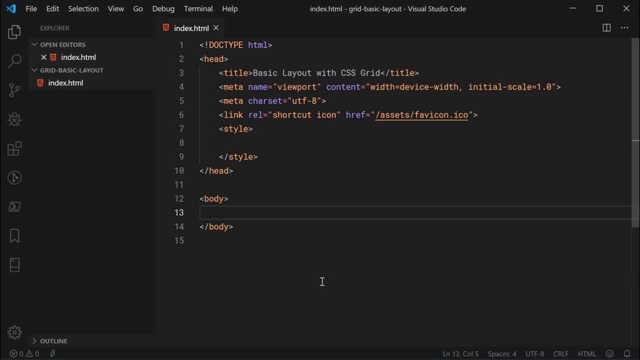 So first, to get started, we need to of course specify HTML. So let's create a container, so a div, with a class of container For the actual grid container. So then inside the CSS, let's just firstly target the body and set a margin of 0 to remove the default margin. this way I can say: container, so target. 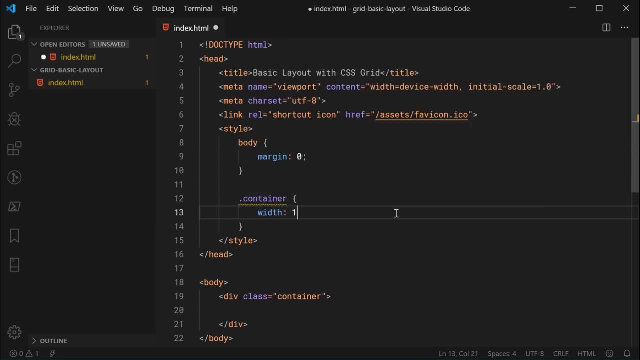 the class of container and say width and make this 100 viewport width and for the height we can say 100 viewport height and of course the combination of these 3 means that the container is going to take up the entire width and height of the web page. So now saving this and refreshing 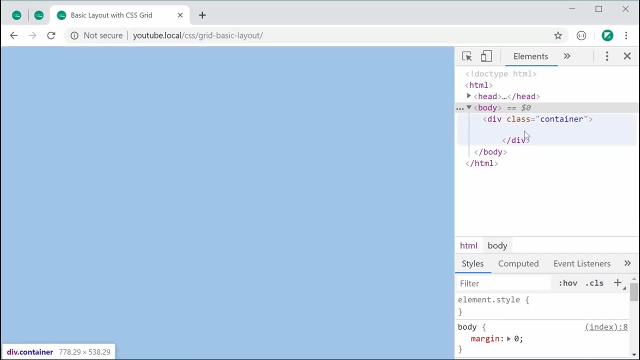 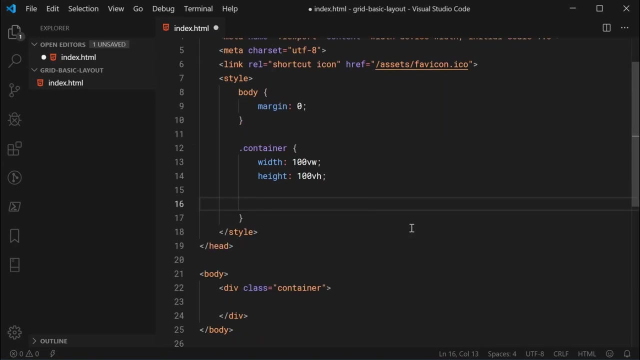 inside the dev tools. if I was to hover over the container, we can see it spans the entire width and the height of the available viewing area. I'm also just going to go back inside here and specify some font styling to make things easier for us to read. So font family. 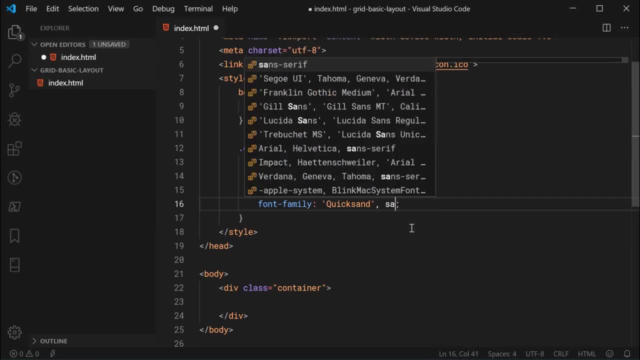 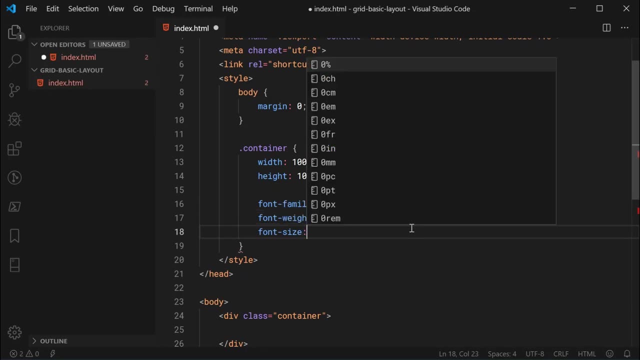 let's make this quick sand with sans serif, And for the font weight, let's make this bold, and also a font size of something like 20 pixels. So now that is all set, So we can now move on to actually using CSS grid. So 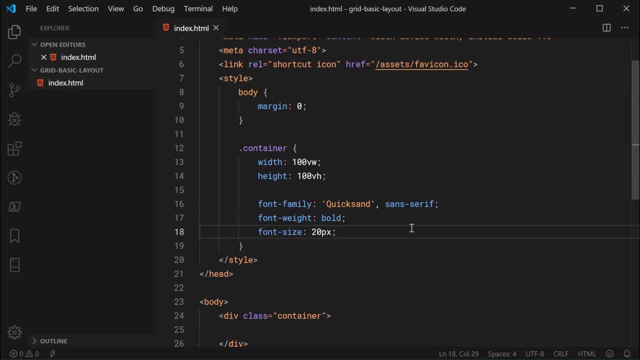 for this we need to firstly specify that our container is going to be a grid or a grid container. For this we can say: display and make this grid. So now we are ready to start adding some grid items, Or at least specify our layer. So now I want to go back to the 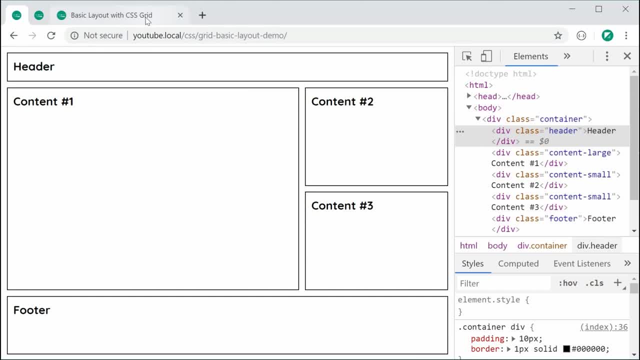 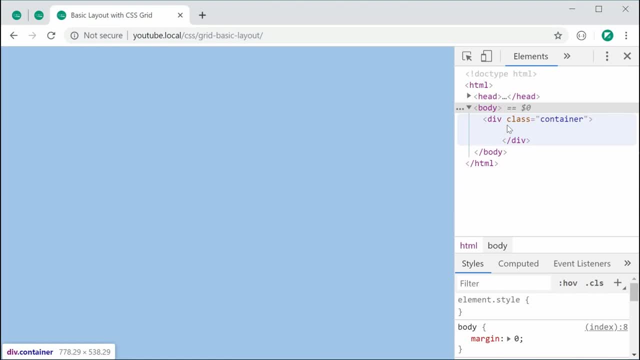 previous layer right here, cause now, of course, our grid right here is ready to actually be used. We need to specify the amount of columns and the amount of rows and also their sizes for our base layer. That's basically how grid works. You have got this base grid layer of. 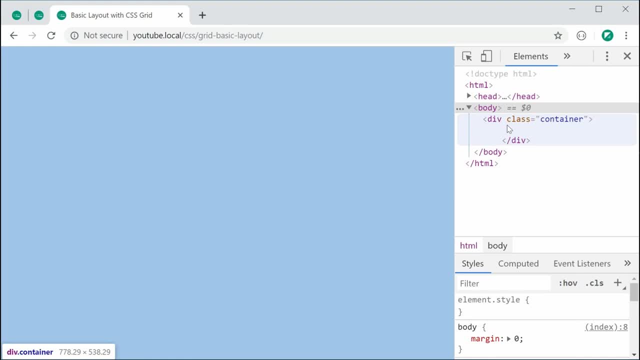 rows and columns in the background, and then, once your layout is complete, you can say that certain elements are going to span multiple rows or multiple columns, or even a combination of the two. So, with that being said, let's go back to this example and analyze and take a look at 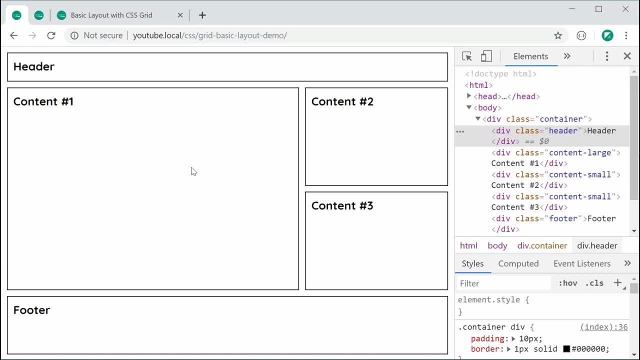 our columns and rows for this layer. As we can see here, in terms of rows, we've got four rows in total. We've got one row, we've got two rows, three rows and then four rows. Even though this content right here is spanning multiple rows, we still consider this to have. 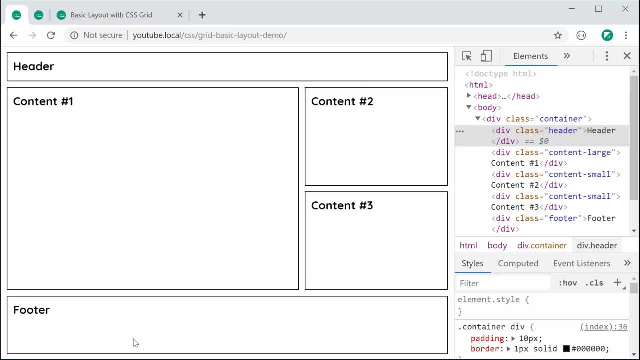 a total of four rows: one, two, three and then four. In terms of columns, this actually has three columns, even though two are visible. We've got one, we've got two and we've got three. That's easier to explain. 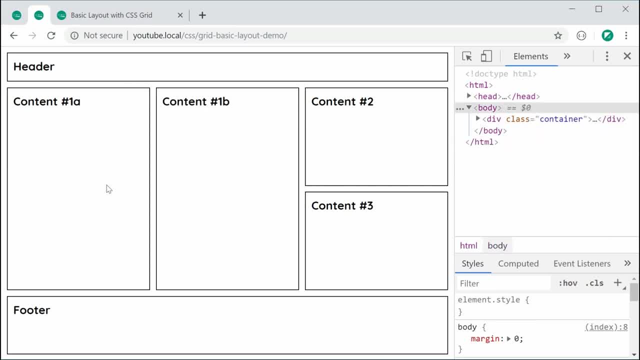 On this example Right here, with the three column layer one, two and three. So, with that being said, this is a four by three layer, which means we can specify this in the CSS for our example, or this right here: 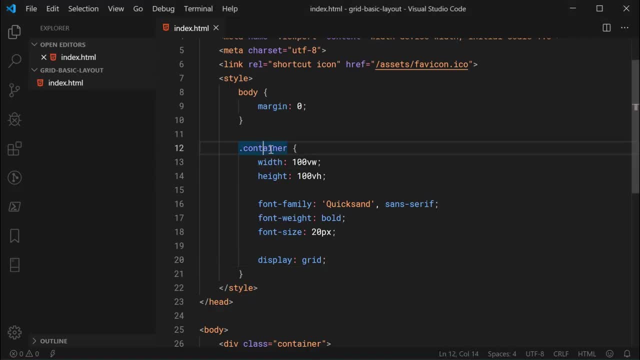 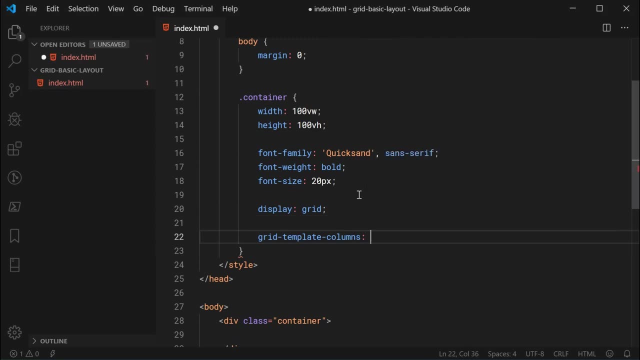 So in the CSS, let's hop inside the container and we're going to say down here GridTemplateColumns, And this right here lets us specify the amount of columns and also their size. So we're going to say one fr, one fr and then one fr. 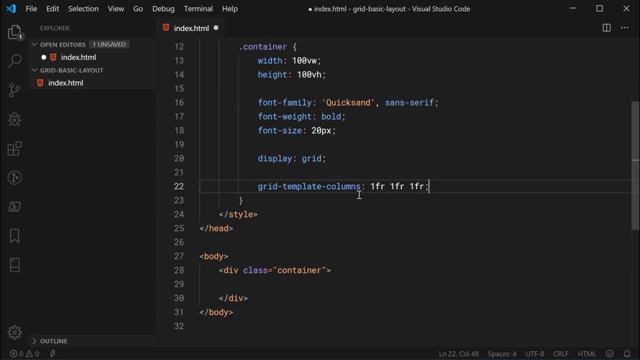 So here we're specifying three columns, since we have three values separated by a space, And the width of those columns is one fraction of the total remaining space. So basically, we've got three evenly spaced columns which are going to shrink in size. 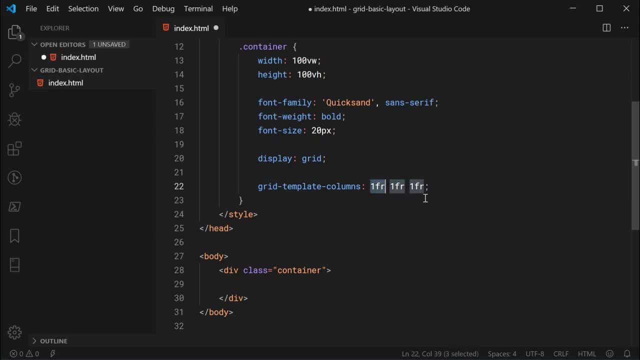 as we shrink our browser, Because it is a fraction, It's going to shrink in size. It's going to shrink in size. It's going to shrink in size Of the available space. Okay, And that is all for the columns. 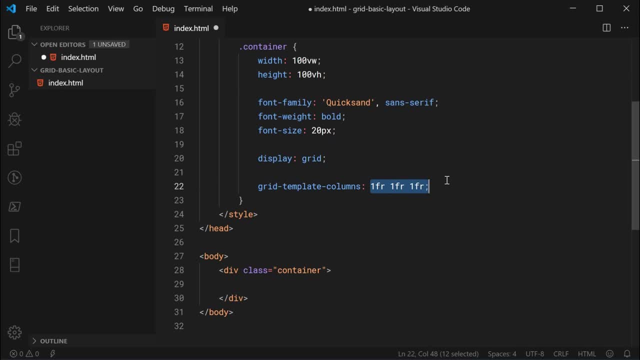 If you wanted to simplify this declaration, you could instead say: repeat, then three and then your value, So one fr. And basically doing this is the exact same as saying one fr, one fr and then one fr. So now we can specify the amount of rows. 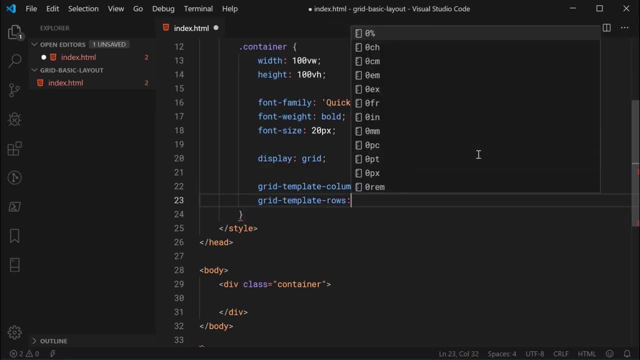 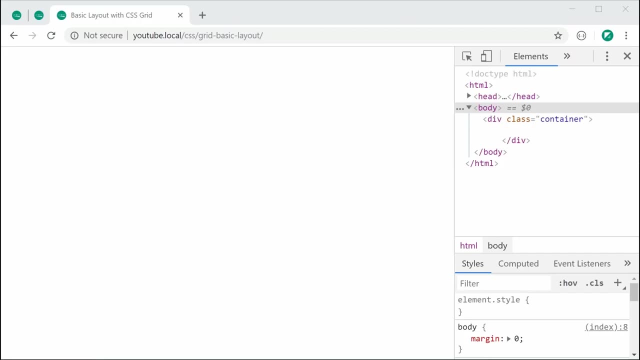 For this we're going to say GridTemplateRows, in a very similar way, And for this it's going to be a bit more complicated, but not too much. So let's go back in the example and we can see right here we've, of course, got the four. 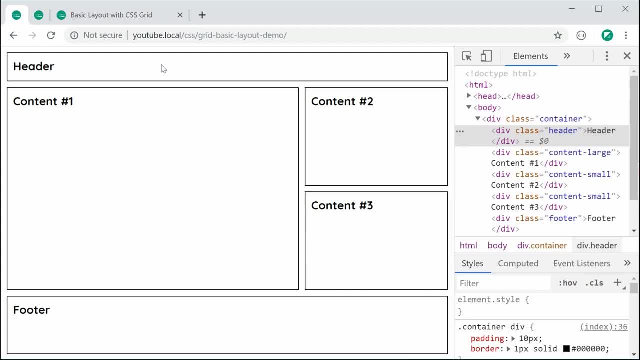 rows. The header row is 50 pixels in height. Okay, These two right here are going to be the same height, but they're going to be once again, a fraction of the available space, And the bottom one here is 100 pixels fixed. 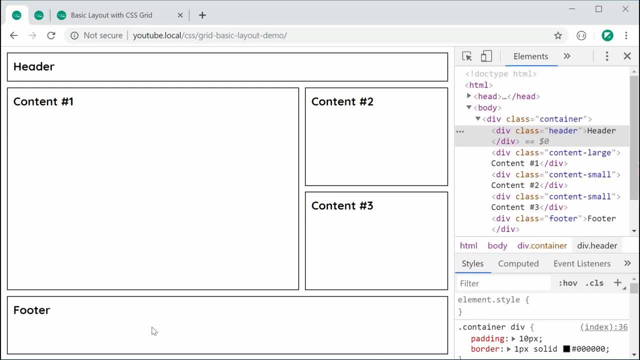 So essentially the top and the bottom are going to be the same height, but they're going to be once again a fraction of the available space, And the bottom one here is 100 pixels fixed And the actual bottom rows are going to be fixed heights of 50 and 100 pixels. 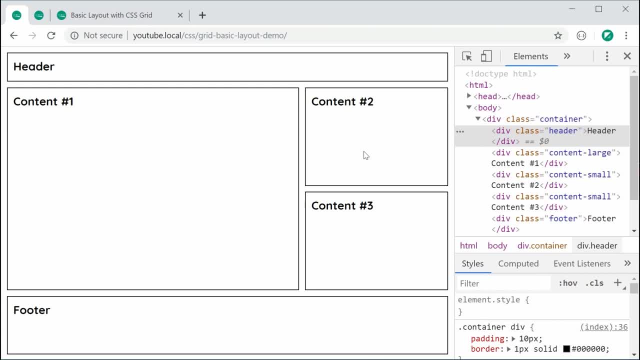 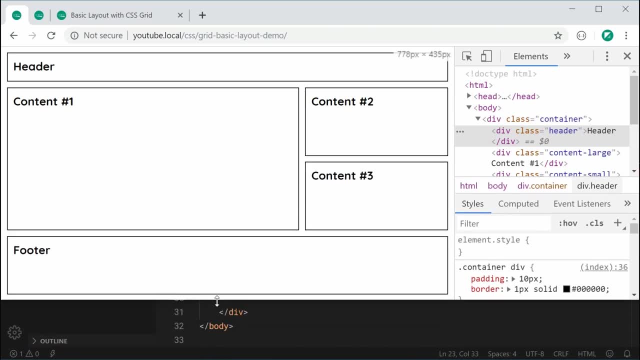 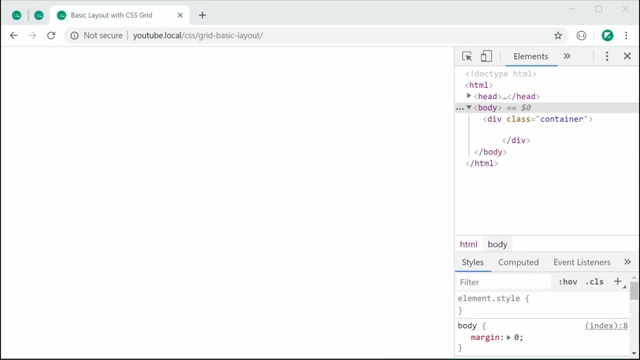 And these two are going to be a fraction of the left or remaining space, which means, if I was to shrink this browser height, we can see that only the two middle rows are changing their height. The header and the footer remain fixed, So for this let's go back inside here. 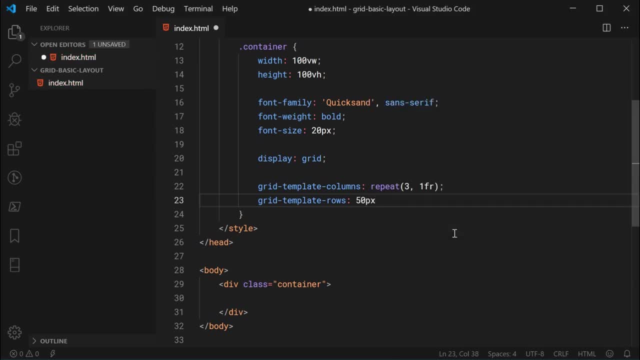 We're going to say 50 pixels for the first row And then one fr, One fr And then 100 pixels for the bottom row. Of course these two are absolute And these two are fractional And they can shrink if they need to when the browser resizes. 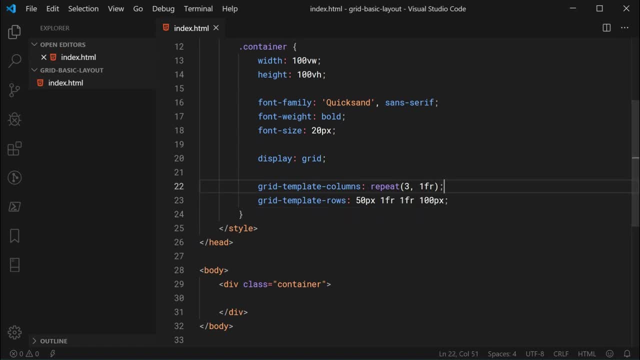 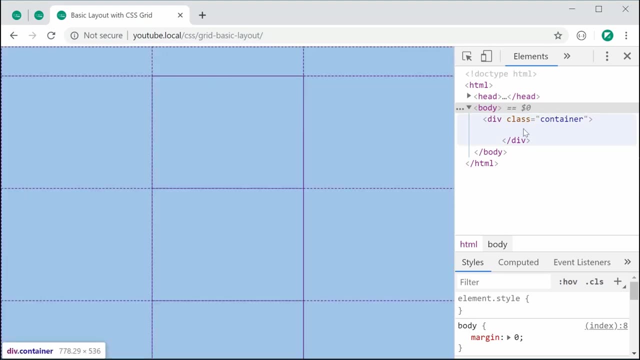 So now we've specified the columns and the rows, I can save this and then refresh the browser Inside the DevTools. if I was to hover over the container, we can see that Chrome gives us a representation of our layer. Of course, we can see that it's not going to be the same size. 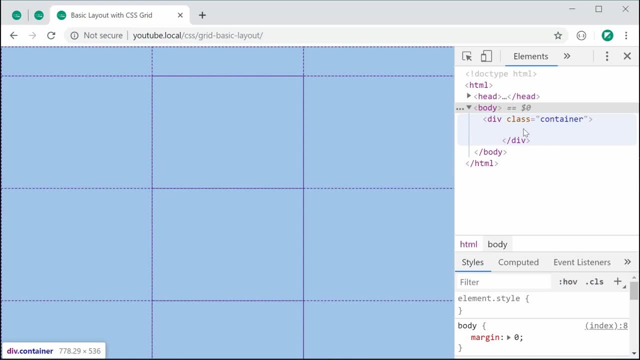 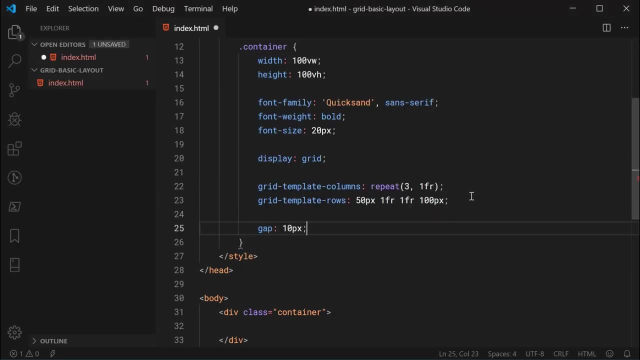 Of course we can see we have all of our rows and columns working perfectly fine. So now we can move on to specifying a gap between each one of our areas here. So for this it is very straightforward: We can simply say gap and make this 10 pixels, for example. 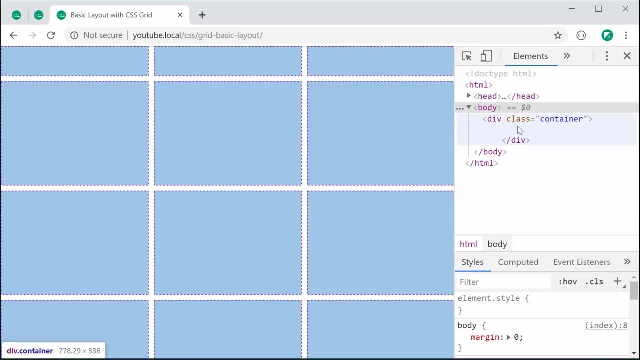 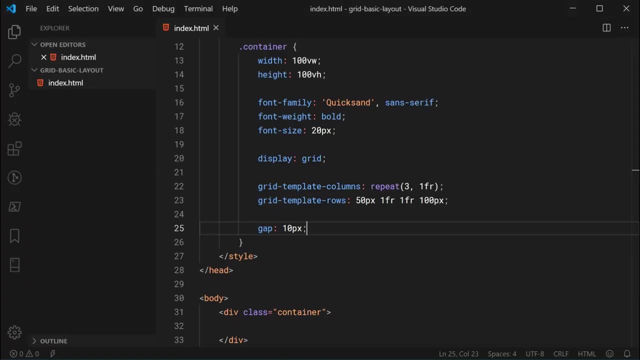 Saving this and refreshing gives us this right here, Of course, a 10 pixels gap, excluding the edges of the container. If you wanted to add a 10 pixels to the container, you could do this. So we can say: padding, make this 10 pixels the same as the actual gap size and box sizing. 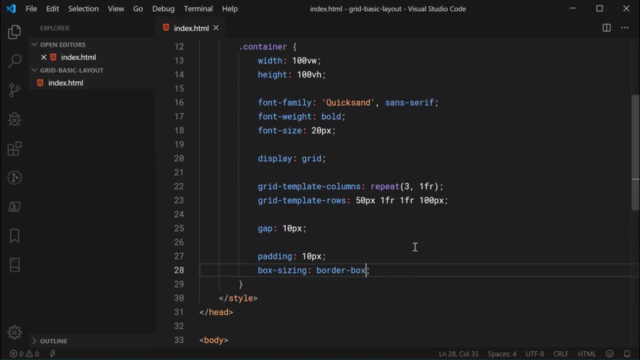 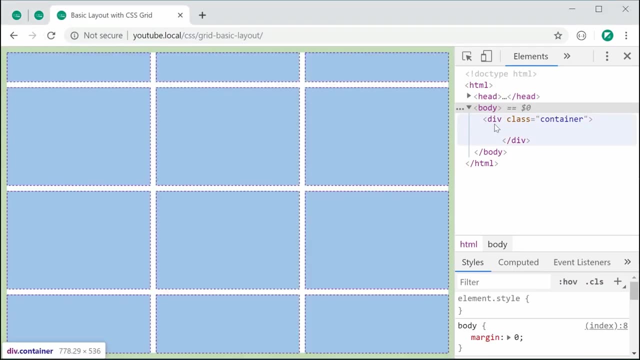 our border box to contain the padding as being part of the total width of the container. Let's save this. and now we have this right here, which is identical to our container in both of these two examples. So now, essentially, we are finished. 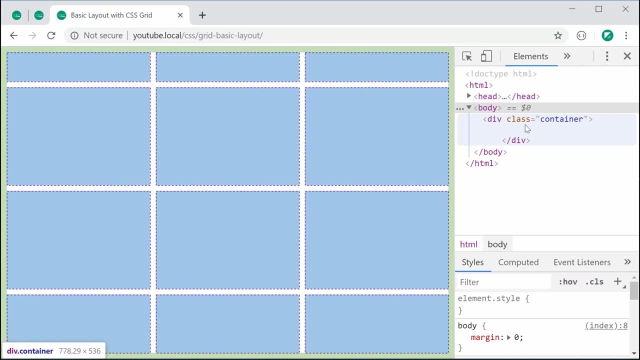 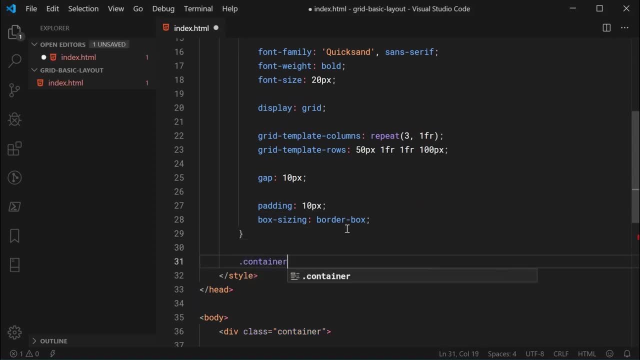 We can save this. We are finished with the container. I do want to go back inside here and just add a new rule set for container and then div. So I'm going to say padding here and make this 10 pixels and say border at 1 pixel solid. 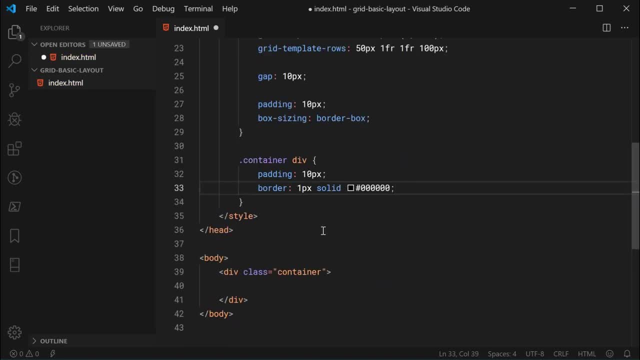 and then black. So now essentially every grid item, so header and all the content and the footer. each one of those divs are going to have a border, So they can actually see how they look, They can see how many rows and columns they span. 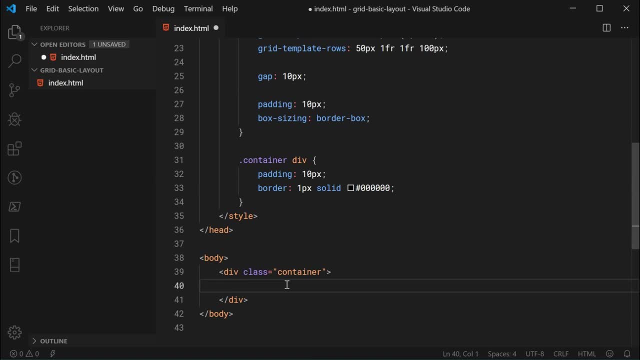 So now let's move on to creating the header. We can make a new div here with a class of header and just say header as the content. So now, if I save this and refresh, we can see that the header is taking up a single. 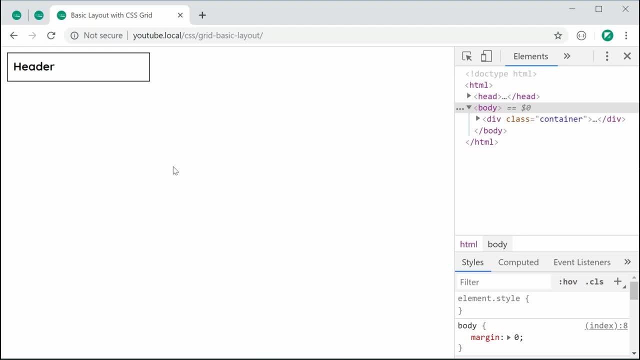 column and a single row in terms of its size. Okay, So to make the header span the remaining rows- sorry, a column. so column number 2 and column number 3.. This can be done using the grid column start and the grid column end properties. So let's go inside here. 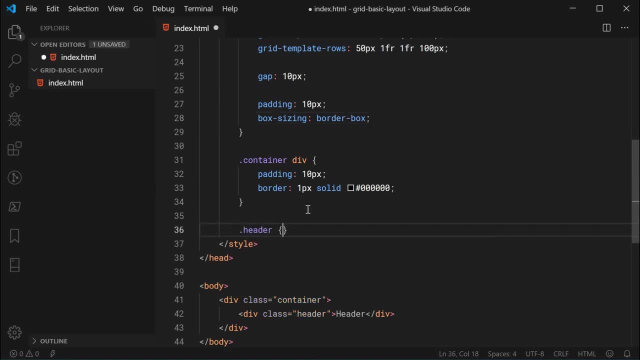 and I'm gonna say for the class of header: grid column, start and make this 1, and say grid column, end and make this 4.. So to explain what the 1 and the 4 means, basically here you're specifying the grid line number, So a grid line. 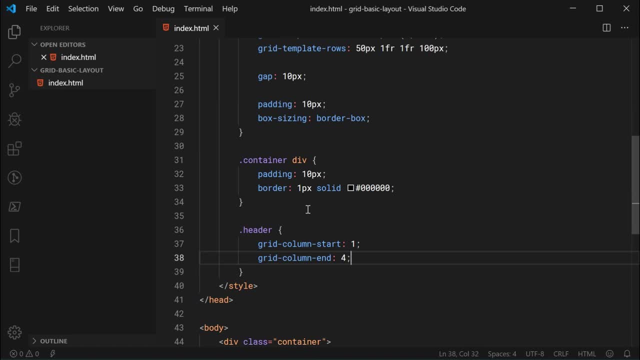 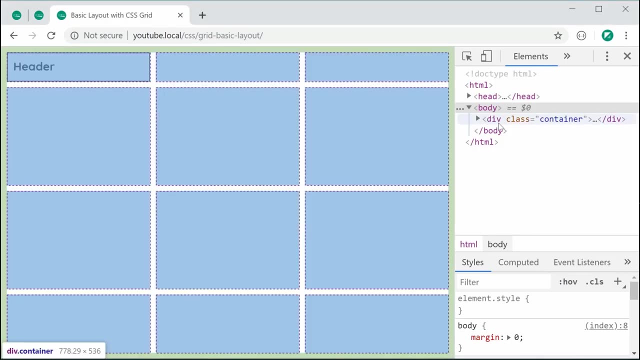 is basically lines between your rows and your columns. So I'm gonna be showing you what that means right now. So in the browser, as we can see here, we've got a total of 4 grid lines on the horizontal- sorry- on the vertical axis We have right here. 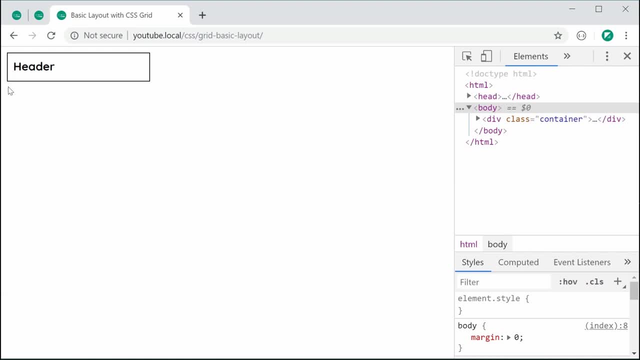 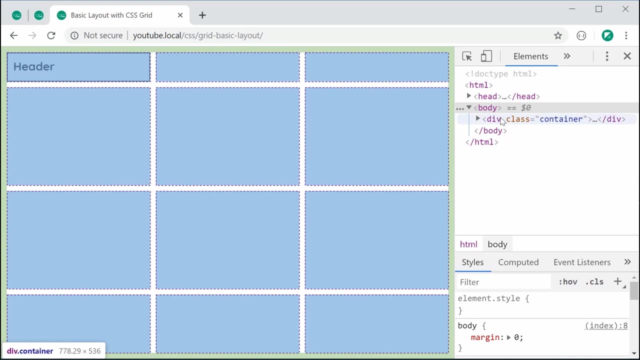 at the edge. this is grid line number 1.. We then have grid line number 2 right here, and then grid line number 3 just about here, and then line number 4, just about here. Okay, That's very important to understand when it comes to making your items span multiple rows or multiple columns. The 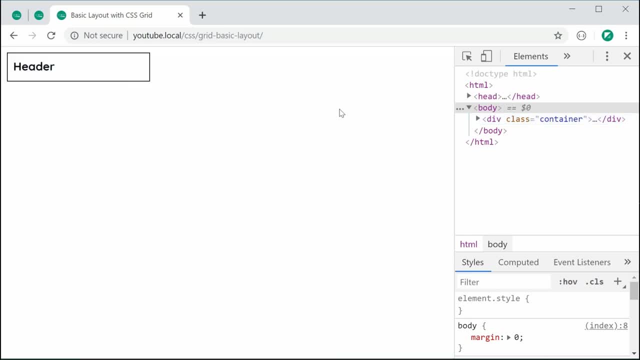 same goes for the horizontal axis. Okay, We of course have grid line number 1 just up here. Okay, Number 2, and then of course number 3, number 5 just down here. So that is what I mean by grid lines. So when I specify grid, 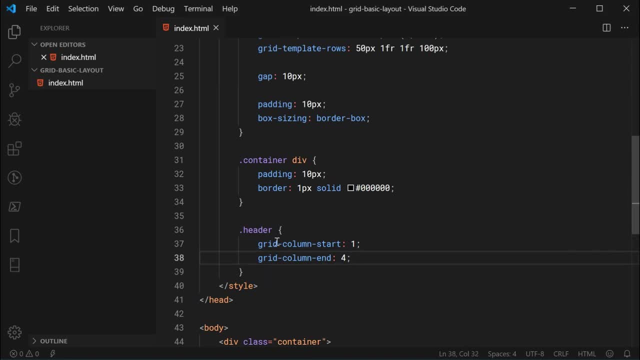 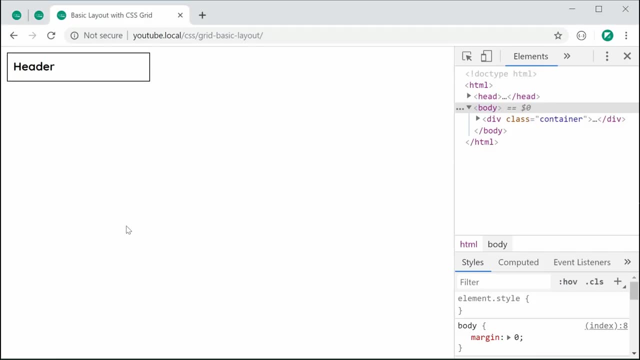 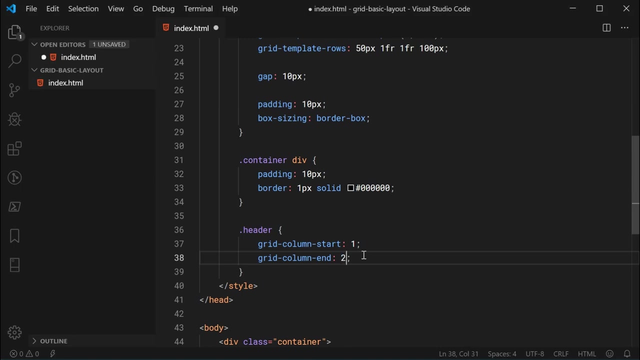 column start at 1 and end of 4, I mean that the header is gonna start at number 1 and finish at number 4.. So now saving this and refreshing gives us this right here For further clarification: if I make this grid column end and say: 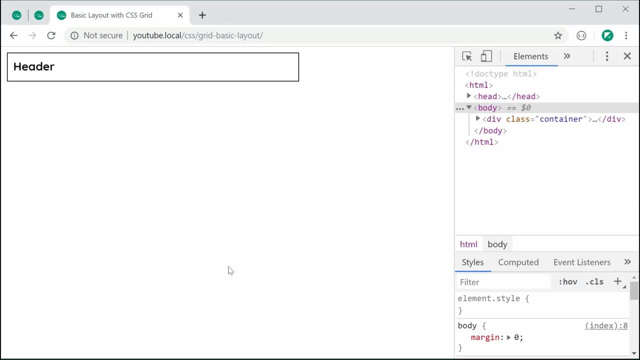 3, save this and refresh. we can see now it goes to 3.. So 1,, 2 and then 3.. Okay, So perfect. So let's just set this back to be 4.. Okay, So now we can move on to creating. 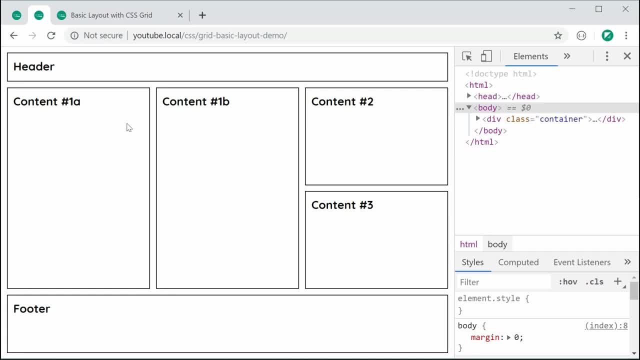 the content right here. So this is where I'm gonna. I'm gonna first show you how to do these two columns for this content, number 1, and then, after that, I'll be showing how to change that so it actually expands, so it actually spans two rows, and then two columns, just like this one. 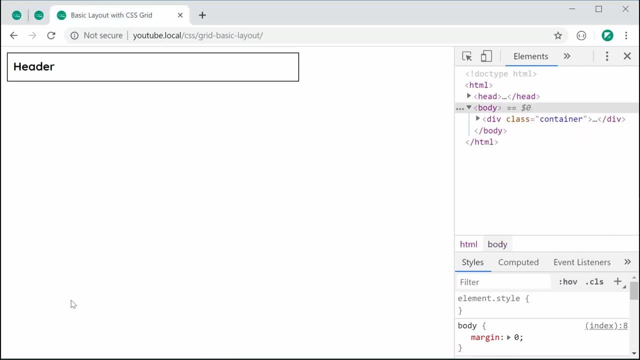 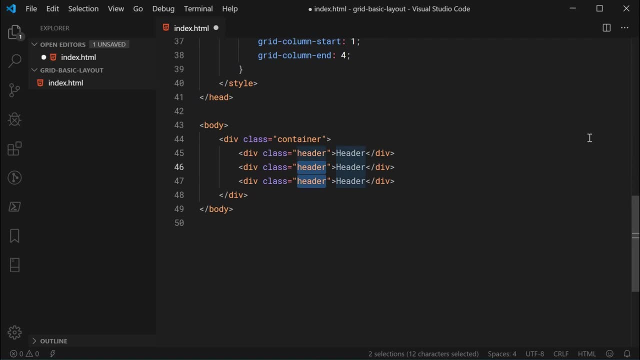 Okay, So back inside here, let's specify two more elements for each one of those content areas. So I can say, right here, a class of content dash large, and we can say, right here, content number 1, and make this A and then make this B. So with this, right here, 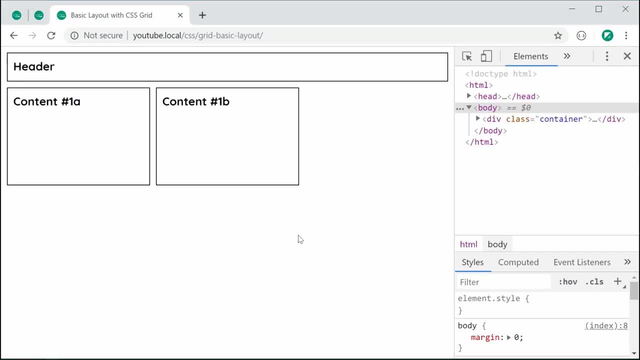 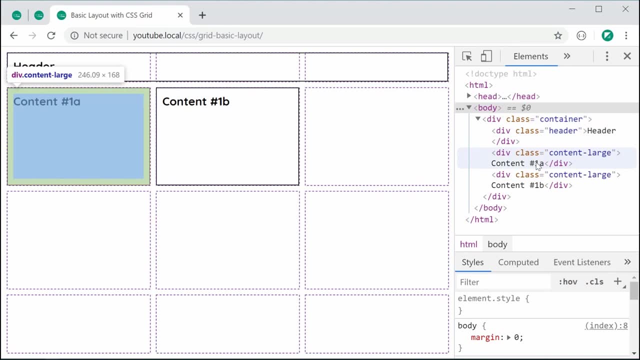 if I save this and refresh, we can see it has successfully flowed across to the second row and the actual items themselves are once again taking up a single piece of area. So a single row and a single column. Okay, So now we're gonna simply, in a very similar way to the header, 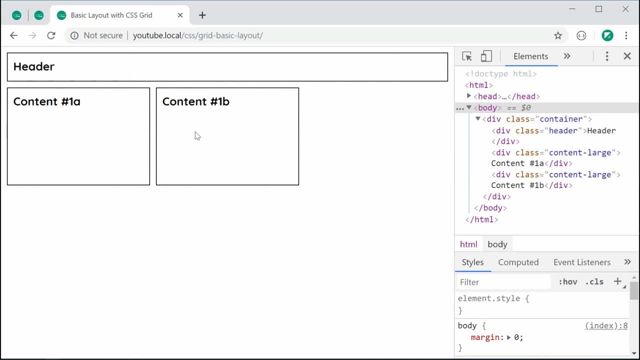 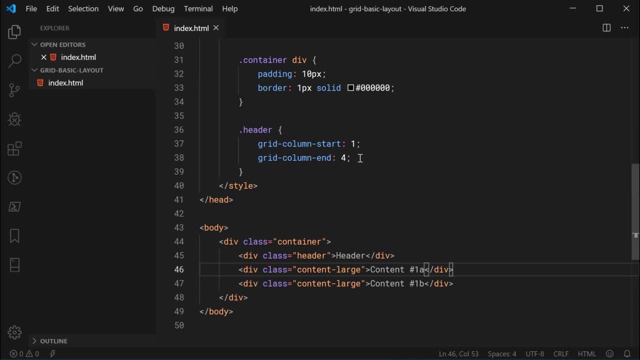 we're gonna make these two span multiple rows, So you may have guessed we're gonna be using the grid row start and the grid row end. to achieve that, Let's target the content large class and make this B So we can make this grid row start. We can make it start, of course, at number 2. 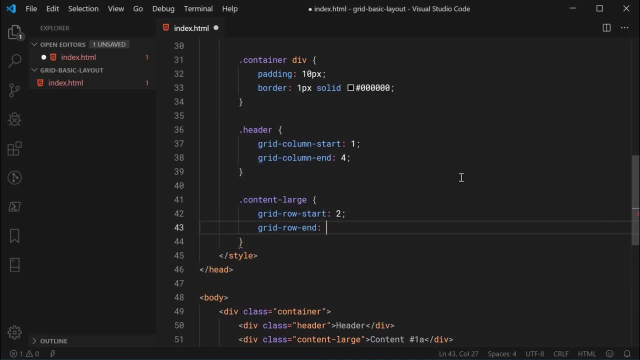 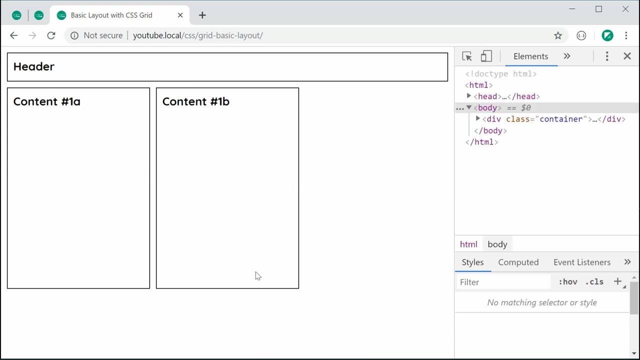 and a grid row end, and this time I'm going to be using span 2.. So basically, span 2 is an alternative to specifying an actual grid line number, And let's just save this and refresh. we can see we get this result right here. 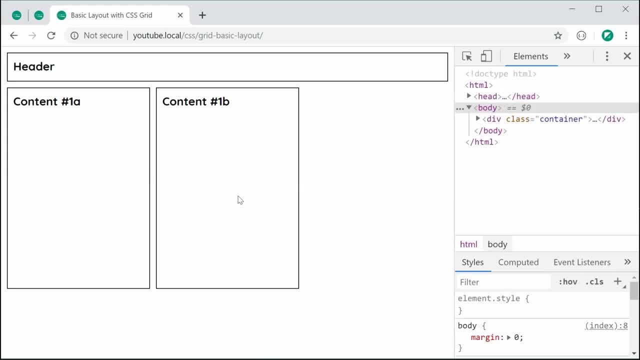 So of course, the grid row start was 2.. So this second grid line right here And we used span. So when I said span 2, it basically means we're going to start here and then span 2 lines. So of course, span. we have line number 3 right here. 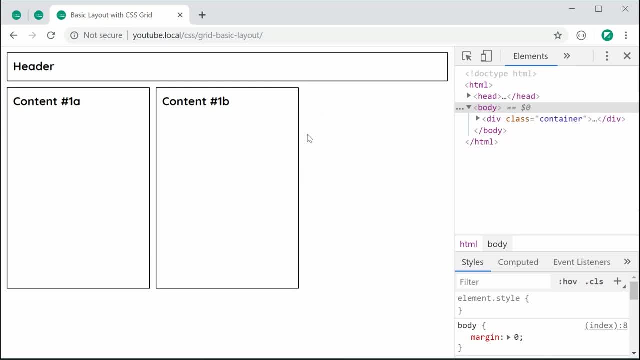 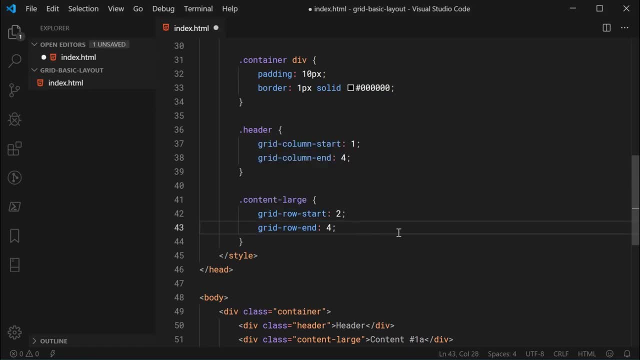 and then line number 4 just down here. So I've started 2 and then span 2 gives us this result right here. Of course, as an alternative, I could simply just say 4.. Instead of using the span 2,. 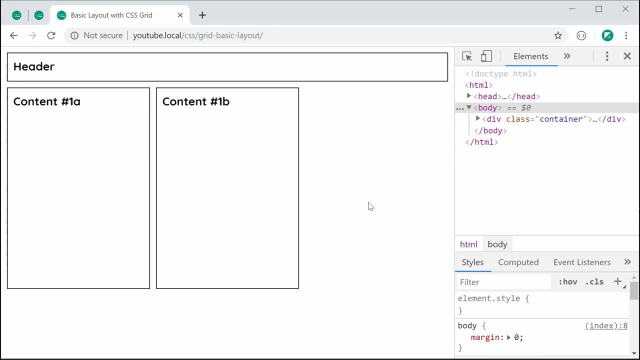 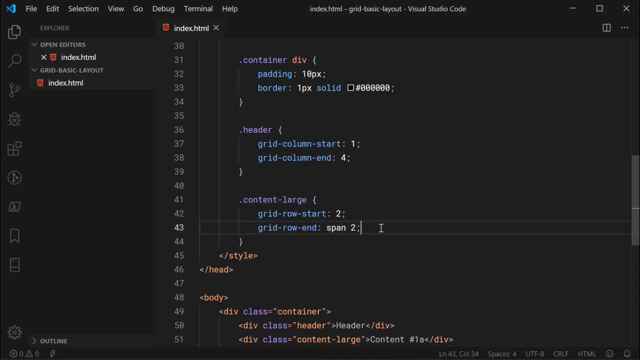 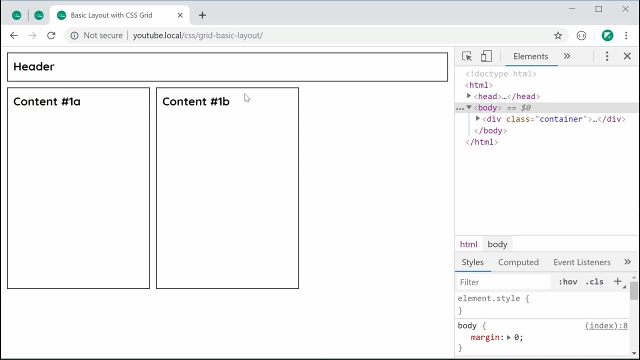 it works the exact same way. Save this, refresh and of course we get no difference. So I'll just set this back to being span 2.. So now, if I want to make this so this single content spans also, you know, this second column here, just like this one. this can be done quite easily. 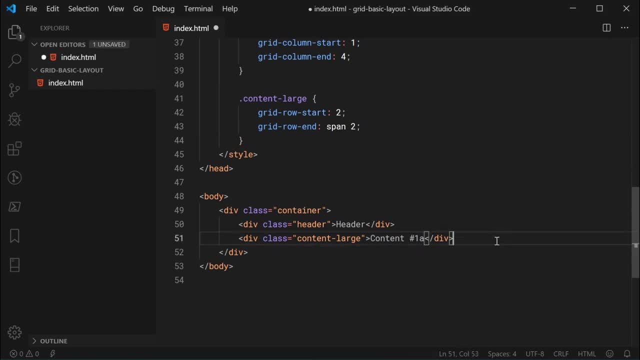 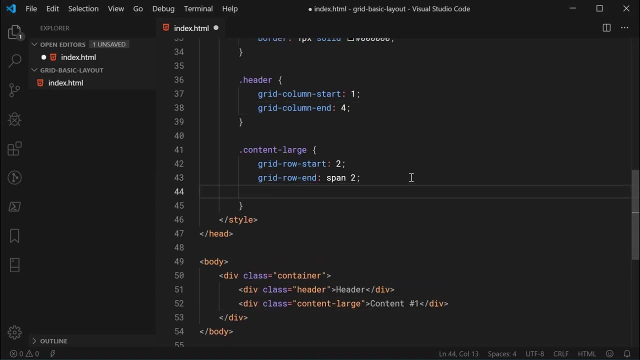 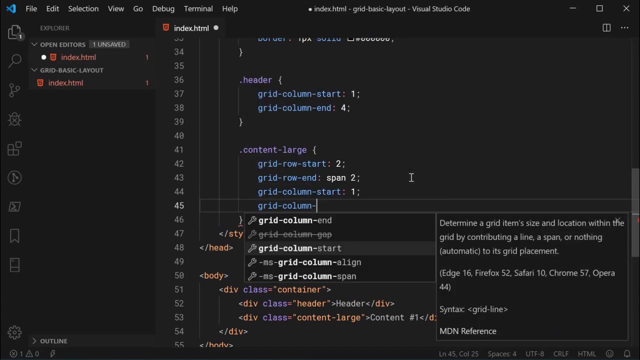 I'm just going to be removing this second content item and making this simply content number 1.. So now we can go inside here and we can also say grid column start and make this 1, and then grid column end and make this 3.. So essentially we're combining both the grid row and the grid. 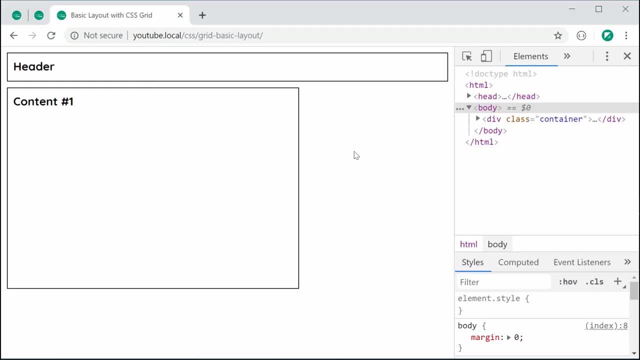 column. So now save this and refresh and we can see right here we start at column number 1 and we finish at column number 3 right here, And of course the row spanning is still in effect. So now we get this large box spanning multiple rows and then 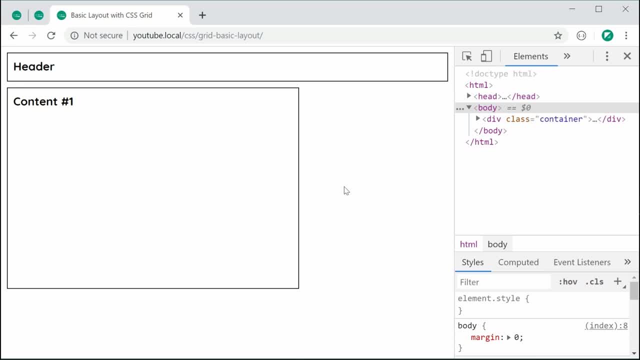 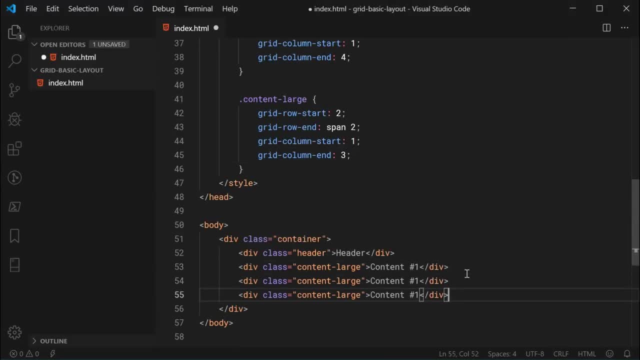 multiple columns. So now, moving on to the tiny boxes on the right side. here, this is going to be very straightforward: We're going to simply create two more elements, So content small and also content small just here, And for this we can say content number 2 and then content number 3.. 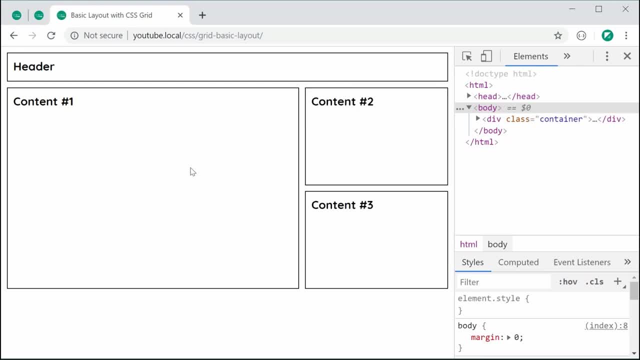 Save this. Of course, these ones also flow naturally, So they're in the correct spot. And that is all for the small content items. So for the footer, it's going to work in the same way as the header, but I'm going to be showing. 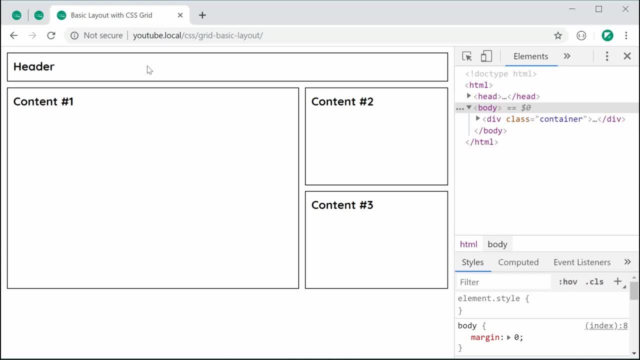 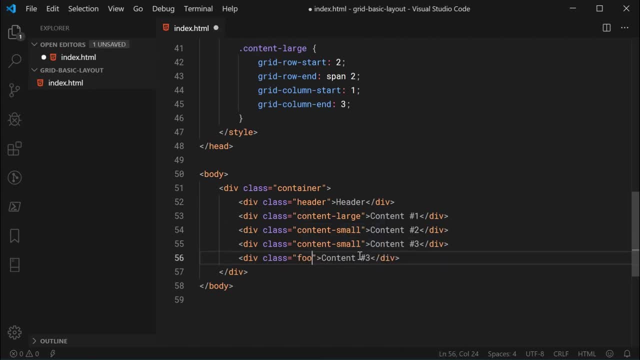 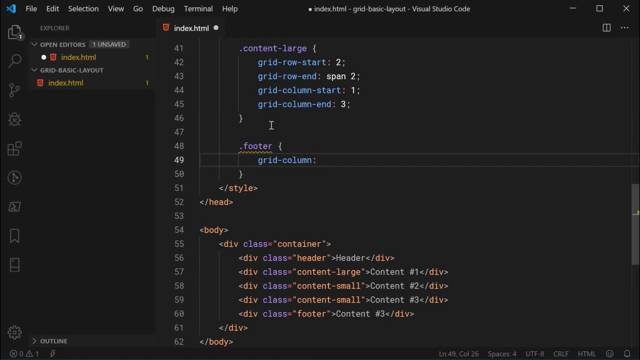 you a different way to specify your column spans. So back inside here, let's create the element for the footer. So with a class of footer just like this, and the CSS rule set for footer is going to say grid, dash column, And then I'm going to say one forward slash and then span 3.. So for this, this is basically. 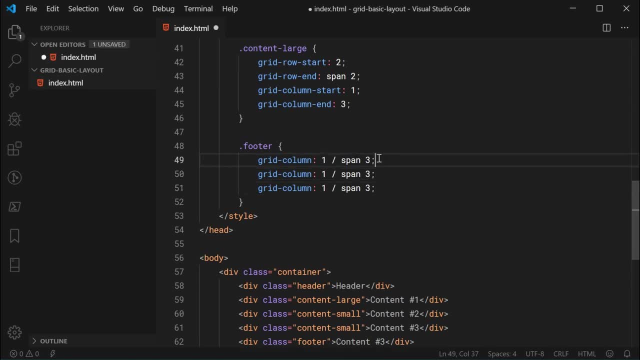 just shorthand for saying grid column start at 1 and grid column end at span 3.. So basically, this right here is the equivalent to this. right here You separate your start and your end with a forward slash. So now saving this. 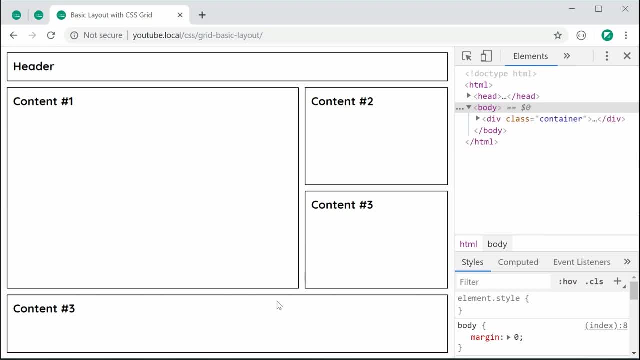 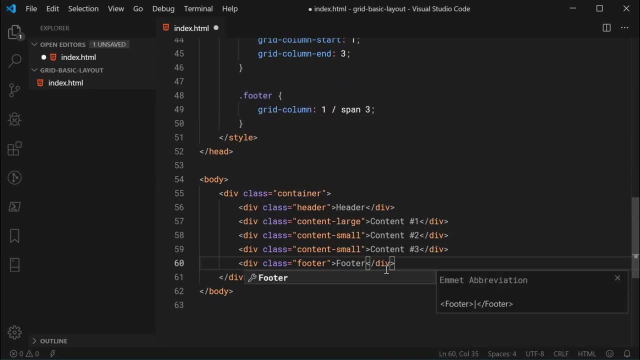 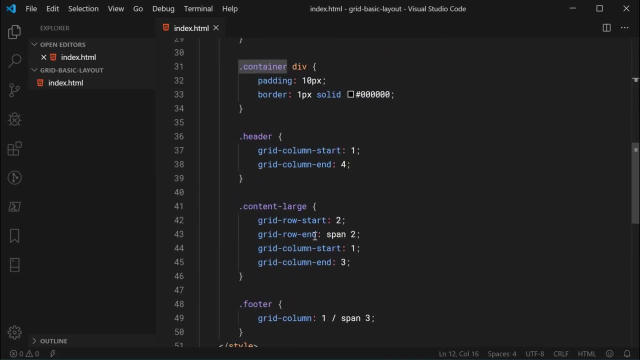 and refreshing is going to give us this result right here, Exactly what we want. I might just go back and make this actually say footer. So one last thing I want to show you is going to be the combination of the grid templates on the container, in a very similar way as